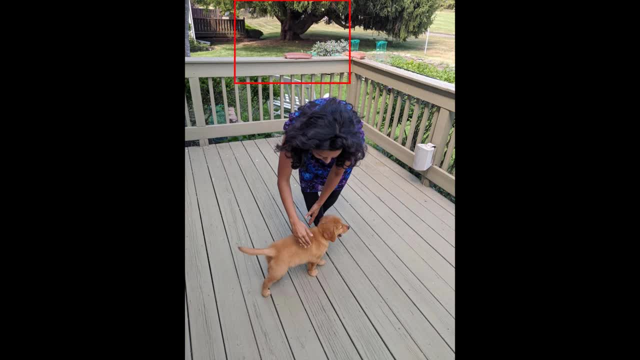 the cropped image within the window, give it to CNN and CNN will tell you if there is a dog in that particular image or not. So you can moving the window horizontally or vertically, one by one, until you get to this point where, for this particular window, your CNN will tell you: this is a 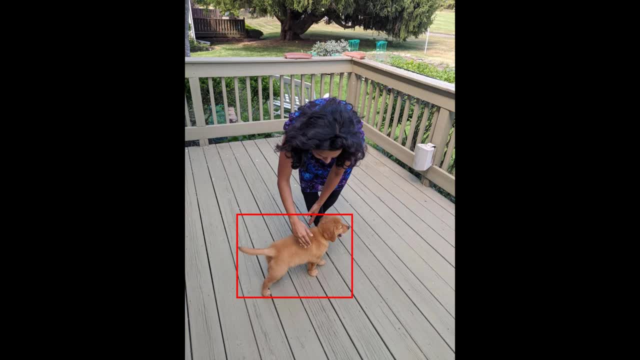 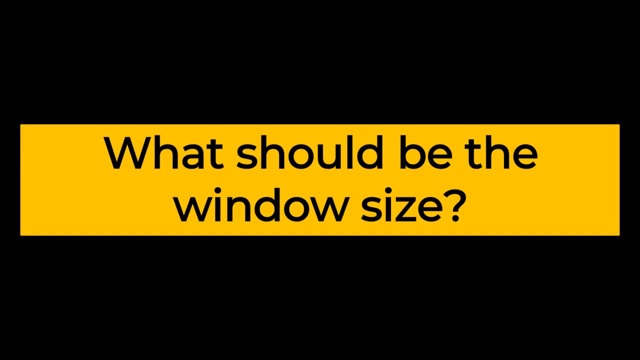 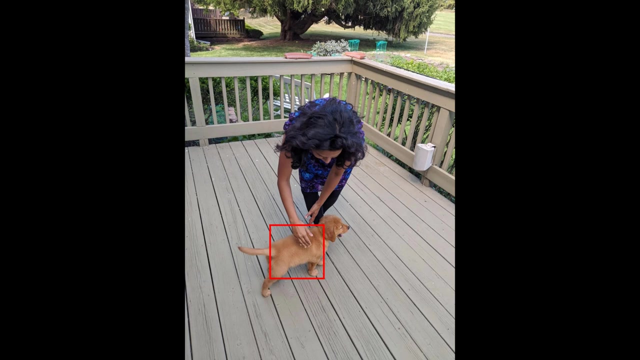 this is a dog. so by doing this sliding window, you can find the location of a dog in a picture. now the question is: what should be the window size? well, trial and error, because let's say, if you start with small window size like this, when you keep on moving this, it might not detect dog. because it's not fitting that. 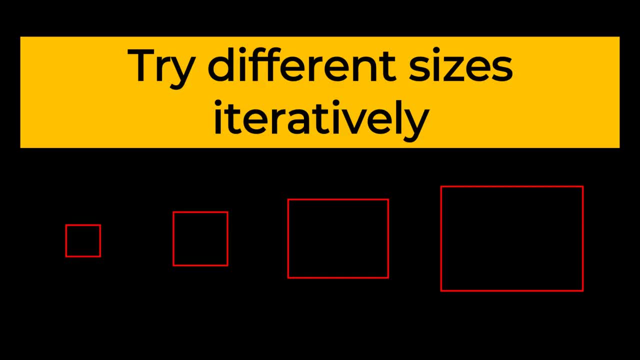 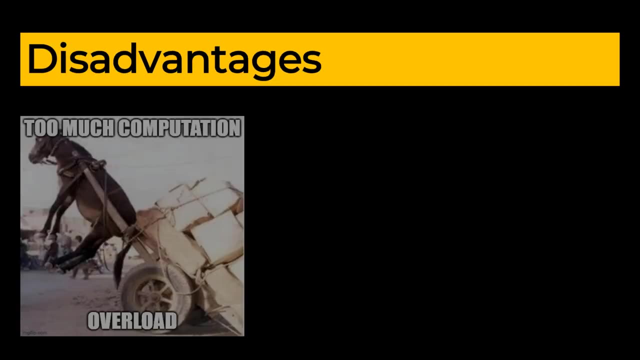 dog object. so idea is you start with a small window, then you increase the window size a little bit, more and more and more, until you find your object. now you can already see the disadvantage of this method, which is there is too much computation. your computer is gonna kill you. 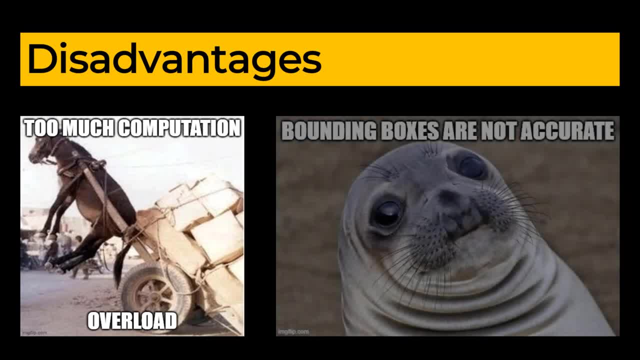 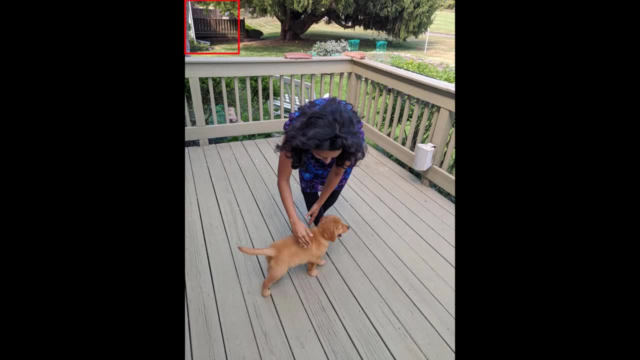 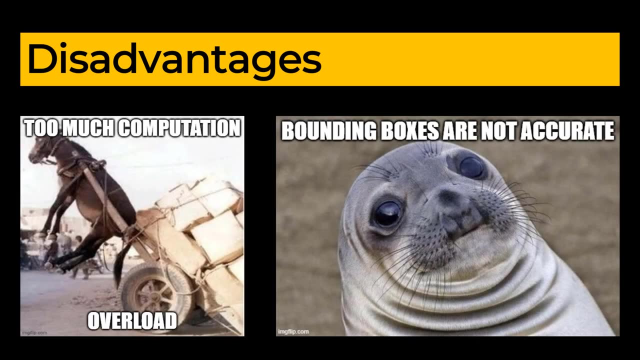 get overloaded, like this donkey, and the bounding boxes might not be accurate. so if your window- let's say windows- are all square, then you might not get this perfect bounding box which is a rectangle. so you don't know whether your object in the image is a rectangle or a square. you don't know. so you're just. 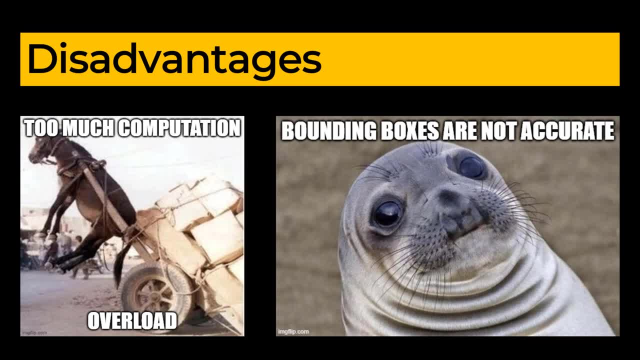 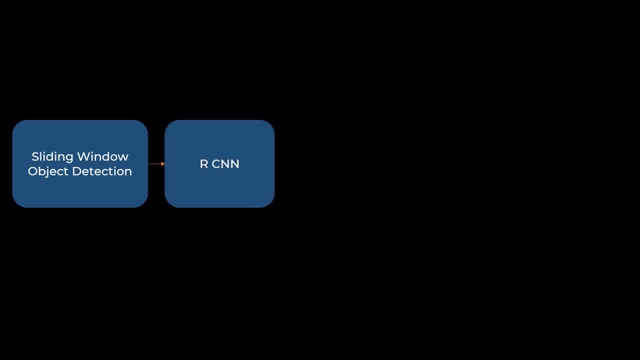 trying it out. so sliding window was a popular technique back in days, but nowadays there are better techniques. as time evolved in the computer vision, there was more research and they come up with a new technique called RCNN, where you propose certain regions for object detection. in the previous case we pretty 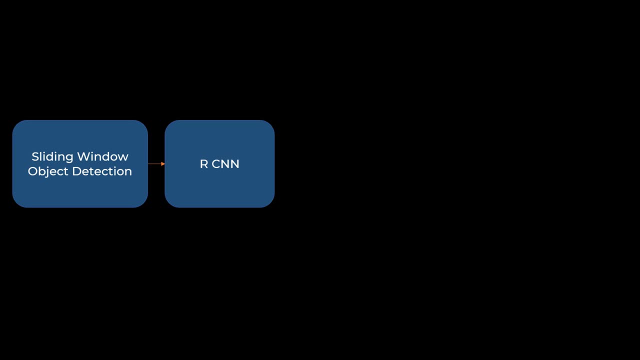 much covered all the image. we tried different region permutation combination, but in RCNN you only try certain area based on image segmentation. you only try certain area based on image segmentation. we are not going to go in in detail, but just think. think of our CNN, as you're.